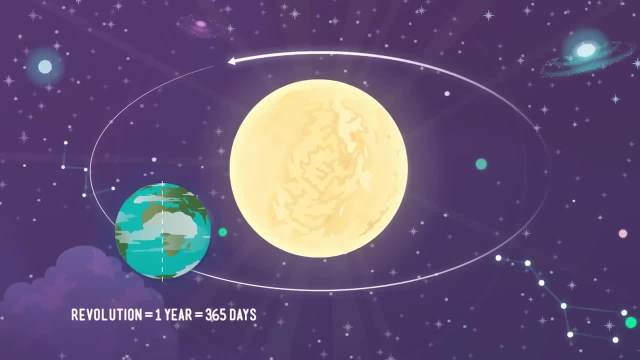 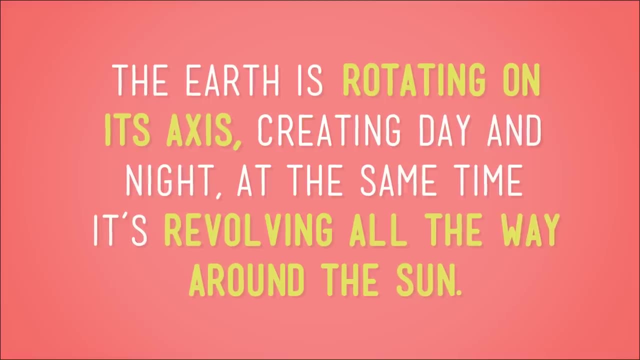 One full orbit all the way around the sun is one revolution, and the earth takes 365 days, or one year, to complete a revolution. So have you got all of this so far? The earth is rotating on its axis, creating day and night, and at the same time, it's revolving all the way around the sun. 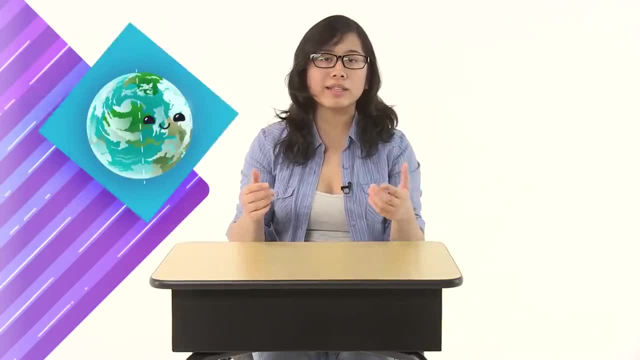 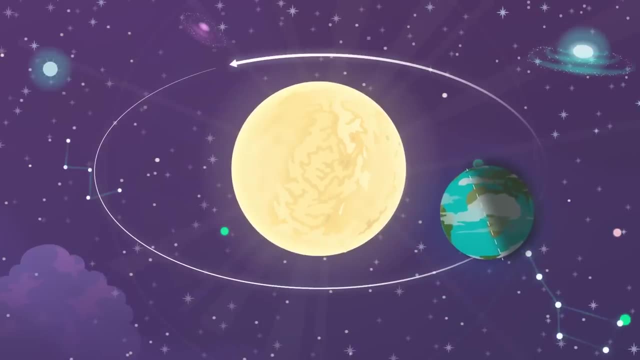 Now here's the thing: As the earth is both rotating and revolving- it's not sitting straight up and down- Its axis is actually tilted just a little. It's not all that much, but this tilt causes one part of the earth to lean towards the sun, while another part of it is leaning away. 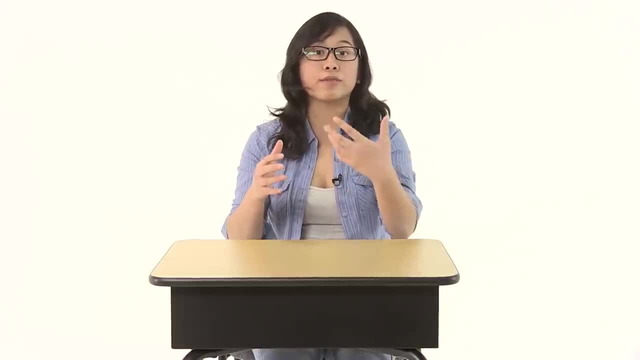 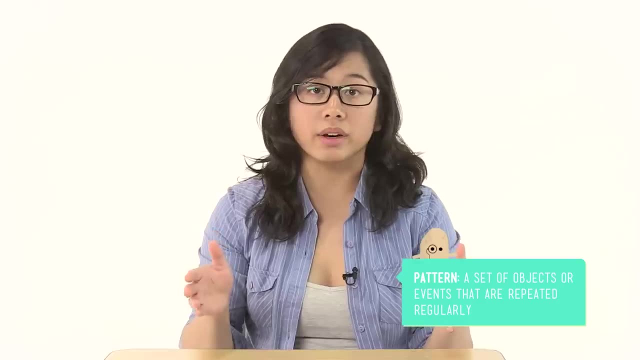 This means that different parts of our planet's surface gets different amounts of sunlight and heat. So why am I telling you all of this? Well, as the earth travels around the sun, it creates a pattern throughout the year. This pattern happens over and over again and I'm sure you've noticed it At certain times of the year. 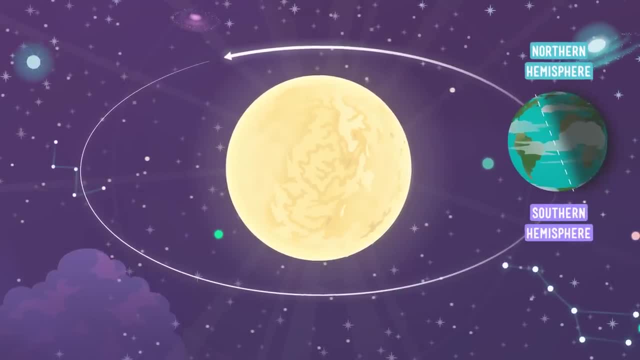 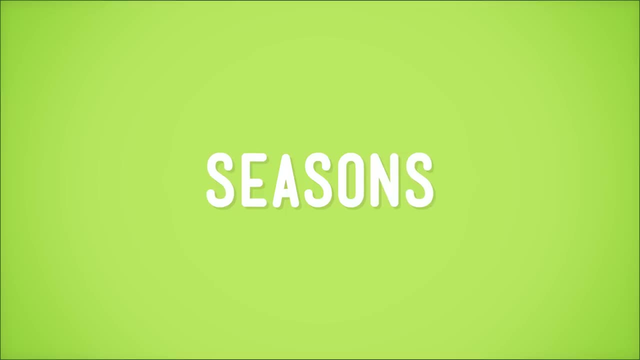 you see, the northern hemisphere leans towards the sun and the southern hemisphere leans away, And at other times, the southern hemisphere leans towards the sun and the northern hemisphere leans away. That pattern, my friend, is what makes seasons When the part of the world that you're living in is leaning towards the sun. 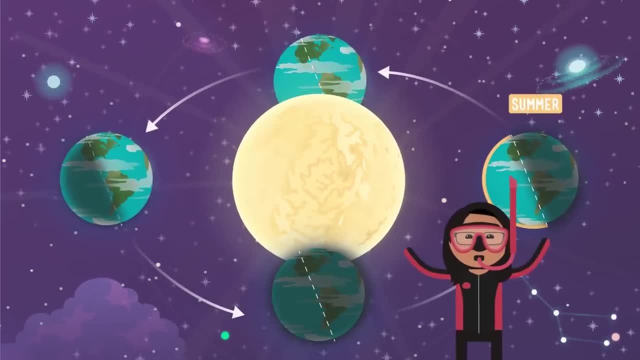 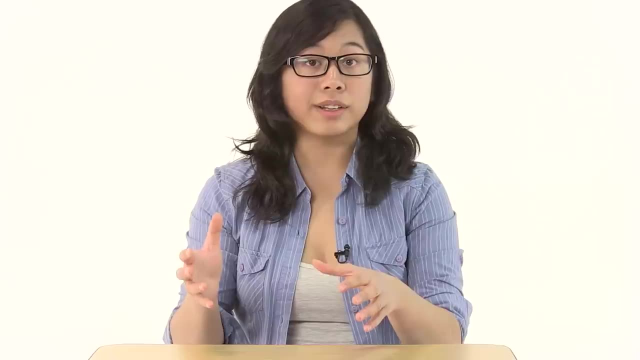 it's warm and the days are long- Summer, When you're on the part that's leaning away from the sun. it's cold and the days are short Winter: In between it's spring or autumn, If the earth weren't tilted. 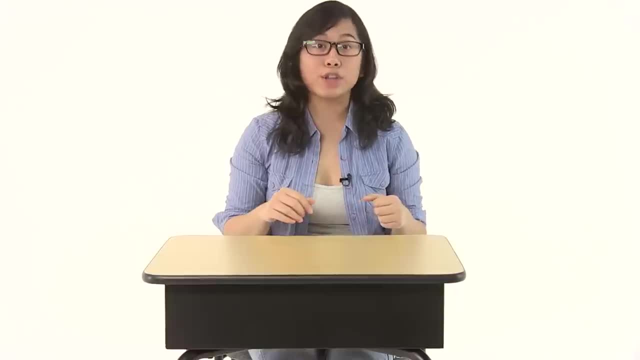 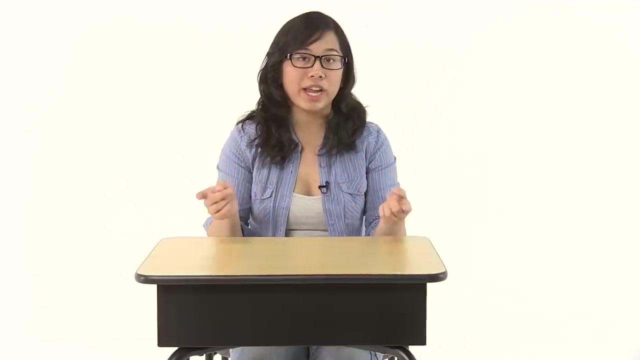 we would have the same season all year long. So, revolution, rotation, orbit: Is your head spinning? Let's do a demonstration to shed a little light on these concepts. Hmm, Okay, you're gonna need a globe and a table lamp without a shade, plus a table to put them both on. 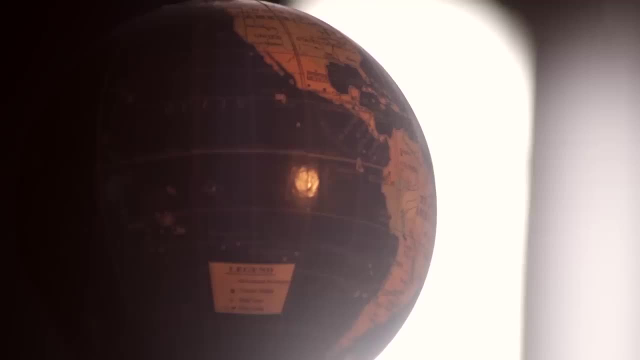 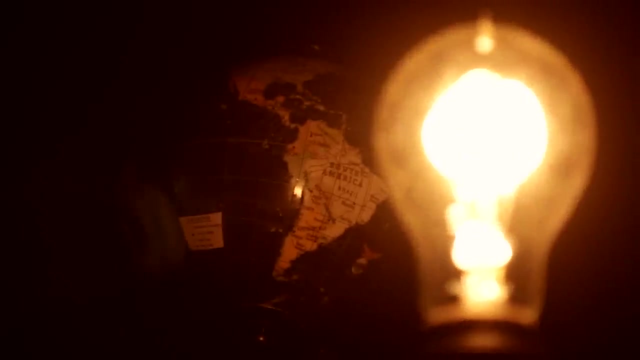 Put the lamp in the center of the table and turn it on. Put the globe on one side of the table. Now hit the lights. The globe is earth. Makes sense, right? The lamp at the center of the table is the sun at the center of the solar system. 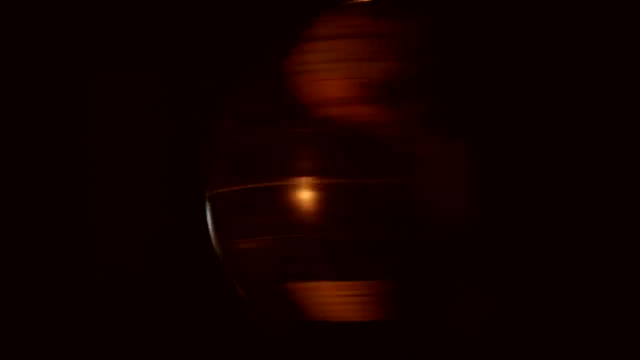 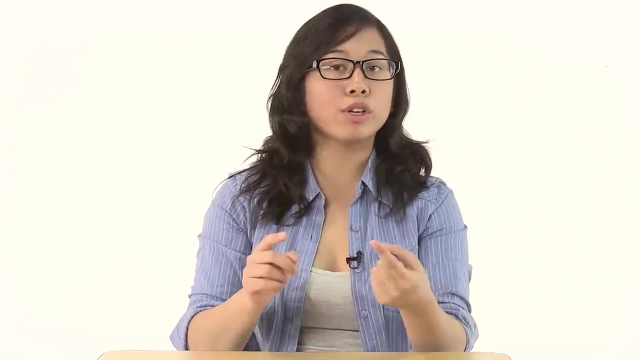 Now slowly spin the globe. As the earth rotates, the sun lights up one side of the planet better than the other. It's day where the light is shining more brightly on the globe and night where it's not. Now let's see what the earth's revolution around the sun looks like. 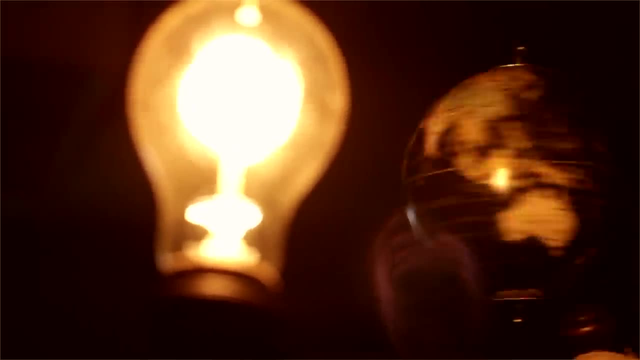 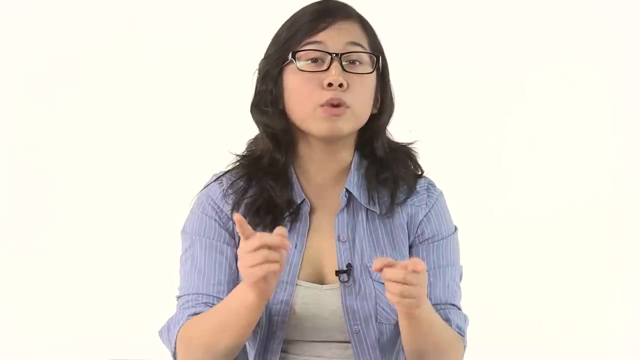 Give the globe a few spins with one hand, while slowly pushing the globe in a circle around the sun Or the lamp with your other hand. So do you notice how the earth keeps rotating as it revolves around the sun? If this were the real sun and earth, by the time you get back to where you started.